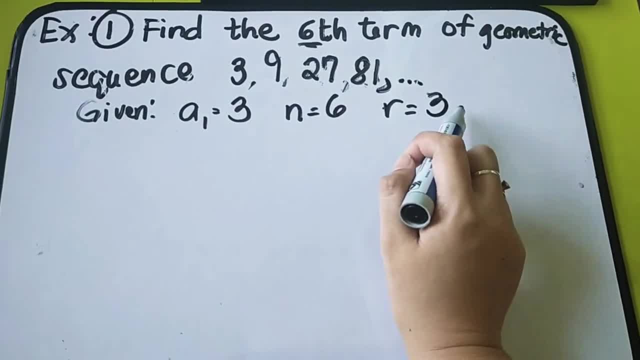 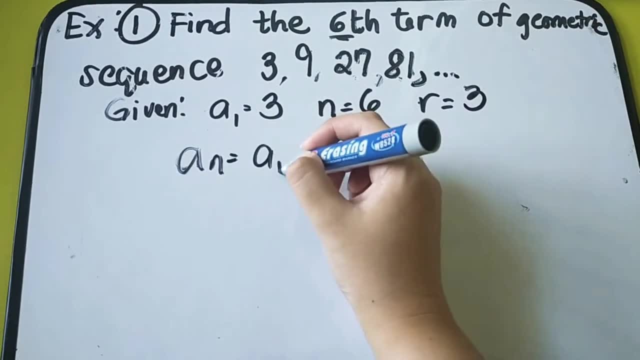 nag-multiply ka by 3.. So that's our common ratio. Again, let us have the formula We have: a sub n is equal to a sub 1 r raised to n minus 1.. So that's our common ratio. Again, let us have the. 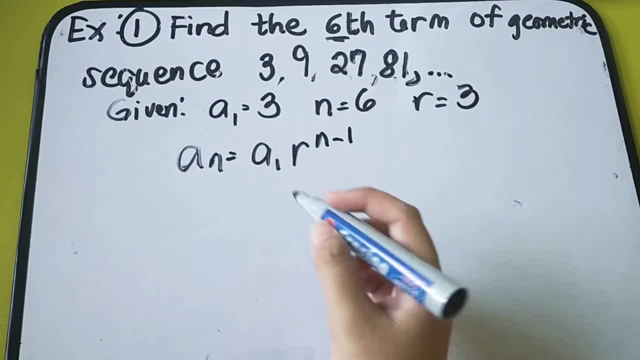 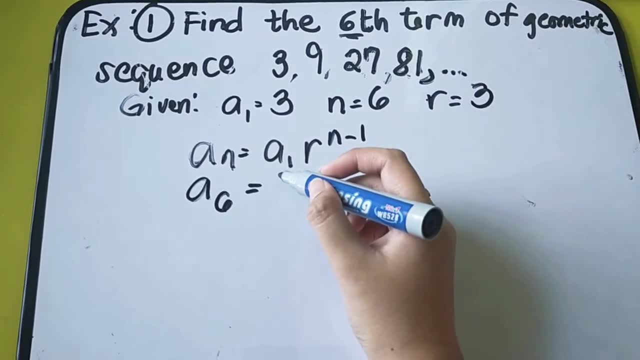 sub n is equal to a sub 1 raised to n minus 1.. So you are going to substitute Palitan ang n A sub. what is n? We have here 6,. equals What is our first term. We have here 3.. Multiplied by what is r. 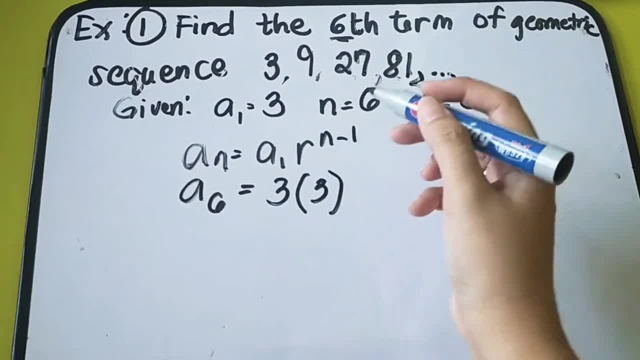 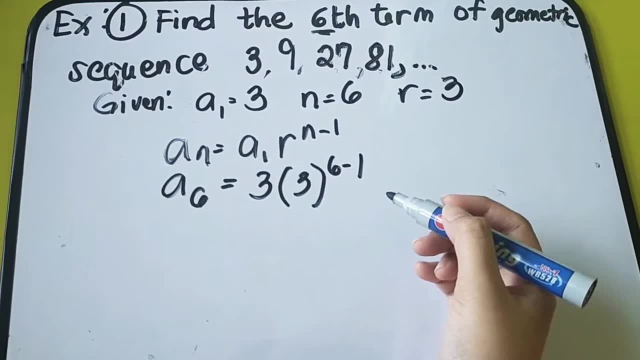 Ang r natin ay si 3.. Then raised to n minus 1, which is 6 minus 1.. Ang n mo ay si 6,. alright, Then anong unang gagawin? Imumultiply mo tong 3 sa 3, or exponent. 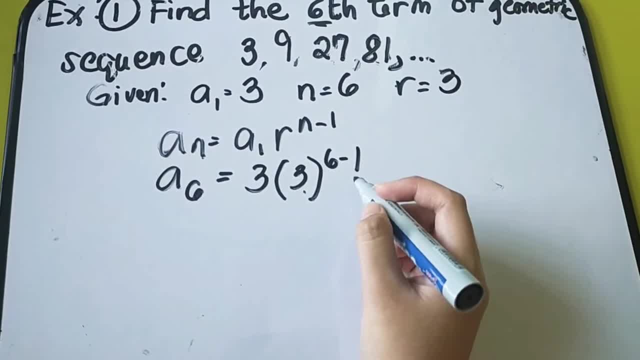 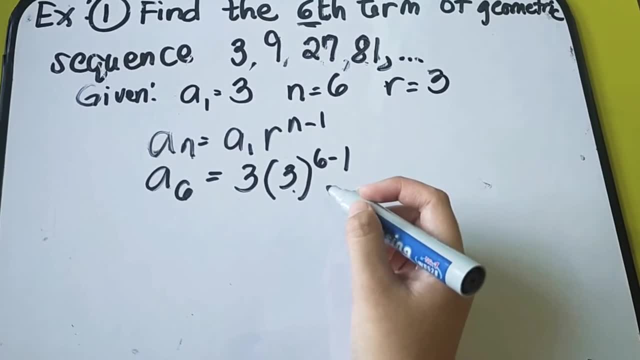 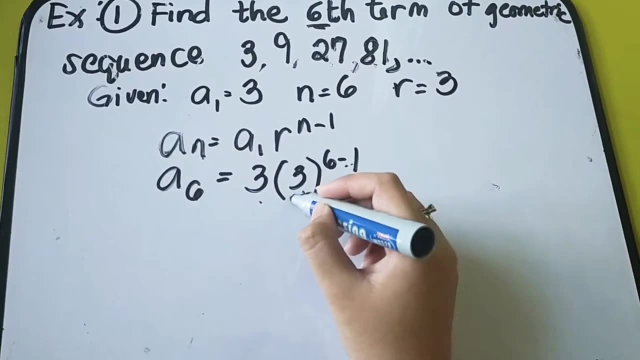 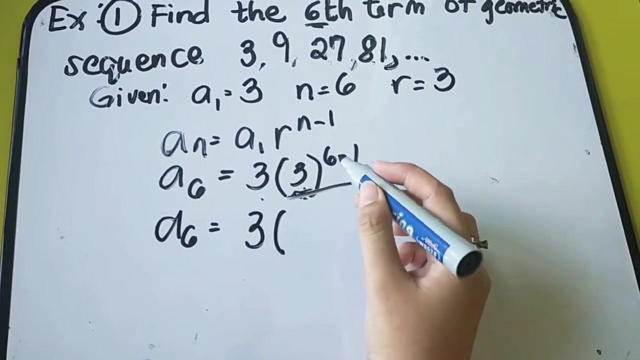 Muna. So syempre PEMDAS rule tayo. Pag sinabing PEMDAS rule, we have parentheses exponent, then MDAS rule na. So dun muna tayo sa exponent bago ka mag-multiply, Is it clear? So lagi yun Exponent muna bago multiply Copy a sub 6.. So we have here 3 times So 6 minus 1 muna 3 raised to 6 minus 1, we have 3 raised to pi. 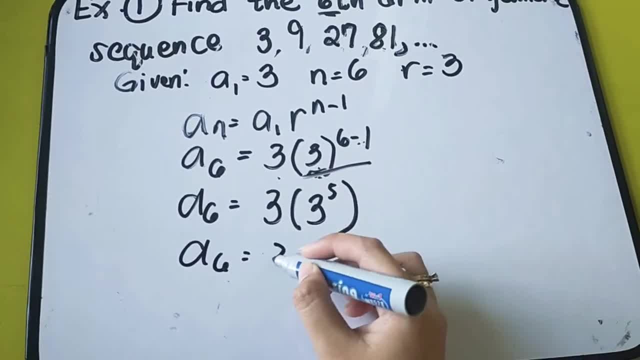 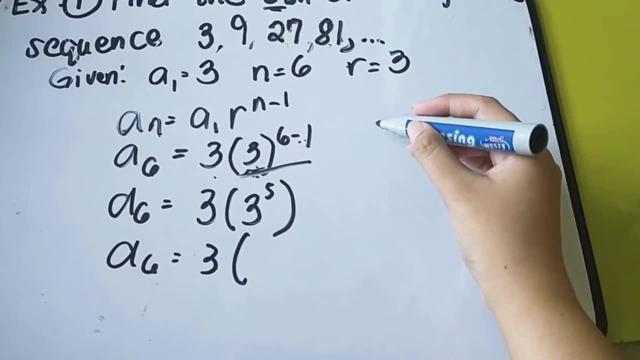 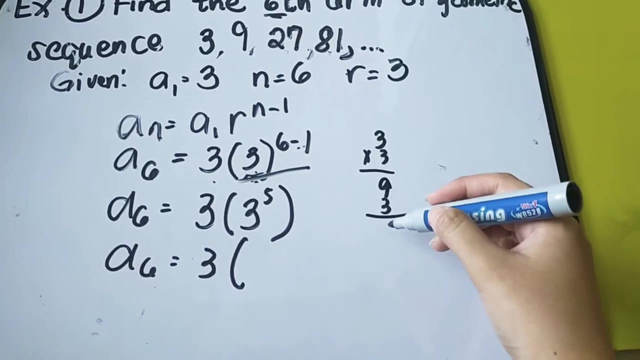 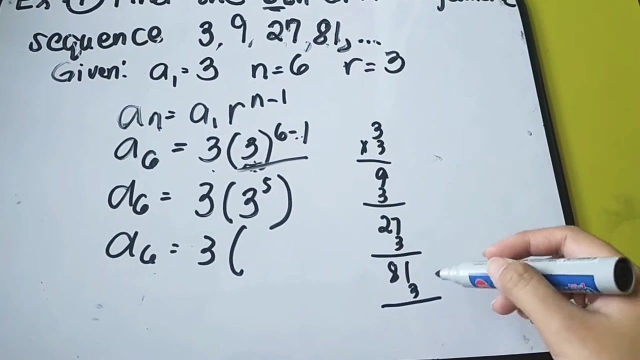 Okay, Then a sub 6 is equals to 3.. Then 3 raised to pi. Paano pag 3 raised to pi, Meaning limang beses mo imumultiply yung 3 sa kanyang sarili, So we have 3 times 3.. Dalawa na to ah. We have 9 times 3 ulit. We have here 27 times 3 ulit. We have here 81 times 3 ulit. We have here 3, we have 24.. 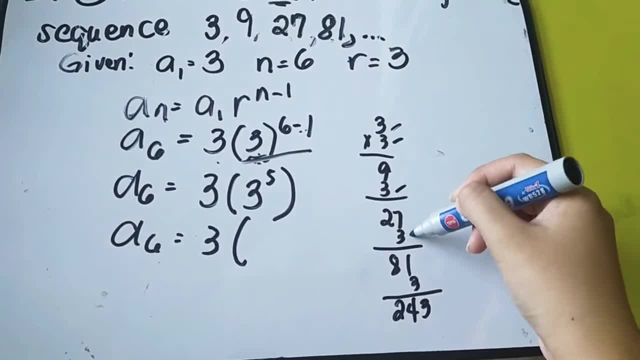 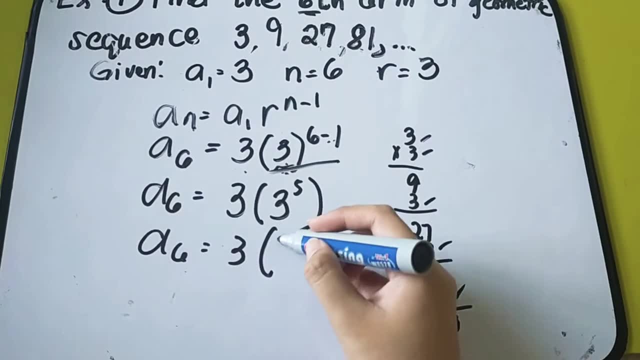 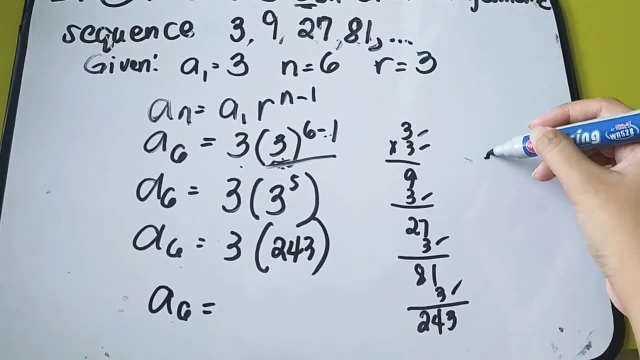 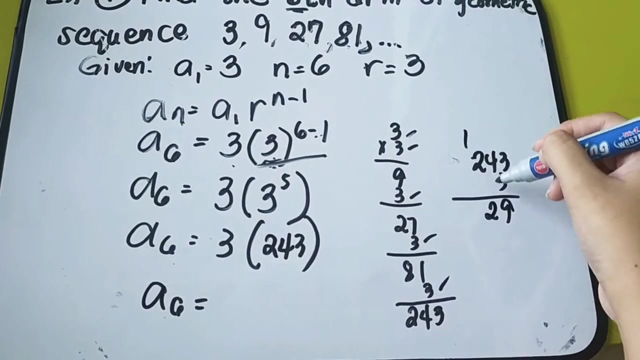 243.. Pabilangin natin 1,, 2,, 3,, 4, 5.. Since nasa bahay ka lang naman, pwede ka namang gumamit ng calculator, ha, We have here 2,, 4, 3.. So we have a sub. 6 is equals to 2,, 4, 3, multiply ulit by 3.. 3 times 3,, we have 9.. We have here 12,. carry 1,, 3, 6, then 7.. So the answer is 726.